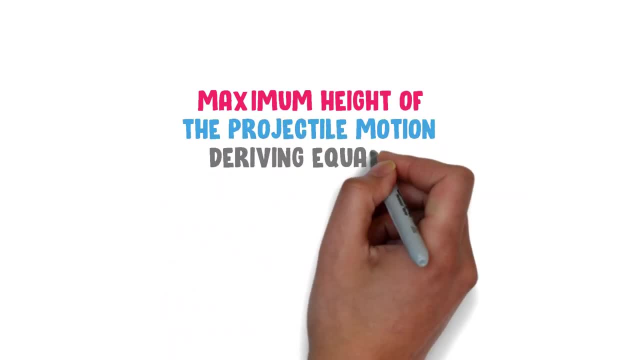 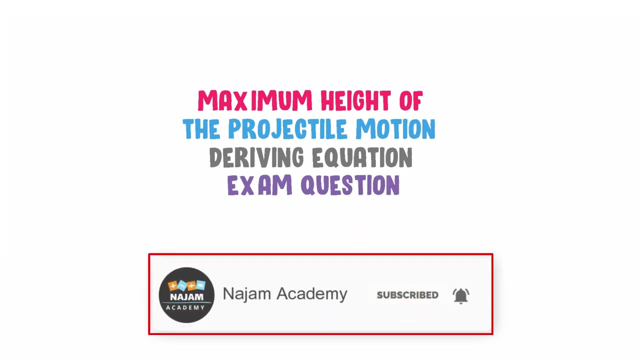 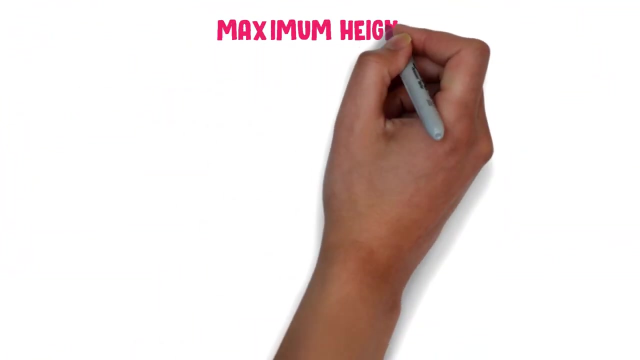 Maximum height of the projectile motion, deriving its equation and exam-based numerical question. Before starting the lecture, click on the subscribe button and get access to our 100 of unique and simple lectures for free Now. what is the maximum height of the projectile motion? 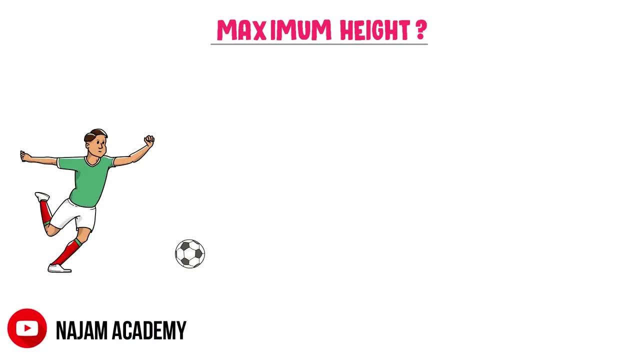 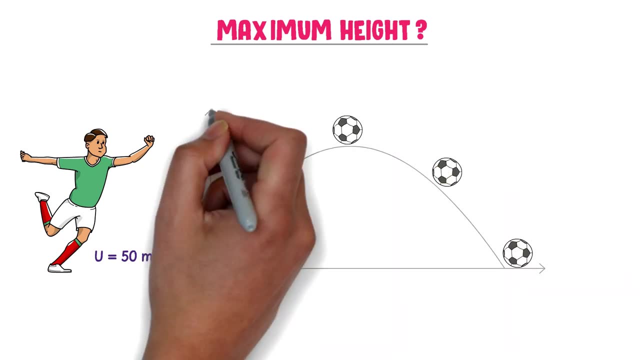 Well, consider a ball. Let you kick this ball and it starts moving with initial velocity of 50 m per second and parabolic path. Let its motion form 30 degree angle with x-axis. Now, this is the vertical position of the ball from the ground. This is also the vertical position of. 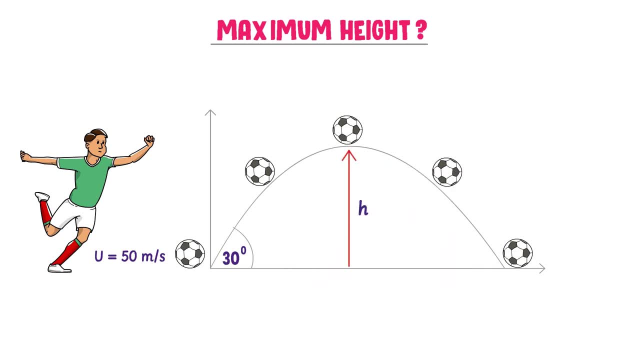 the ball from the ground, But this is the highest vertical position of the ball from the ground. From this point onward, the ball falls down. Thus, this highest vertical position of the ball is known as a maximum height of the projectile. Therefore, we define the maximum height of the projectile as the highest vertical position of. 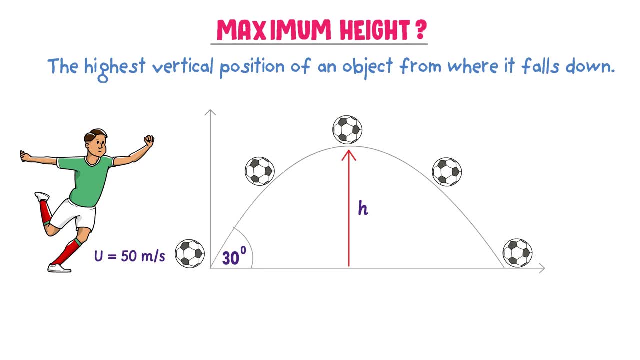 the object from where it falls down is called the maximum height of the projectile. Let me repeat it: The highest vertical position of the object from where it falls down is called the maximum height of the projectile. Now, in the first part of projectile motion, we learn that this ball moves. 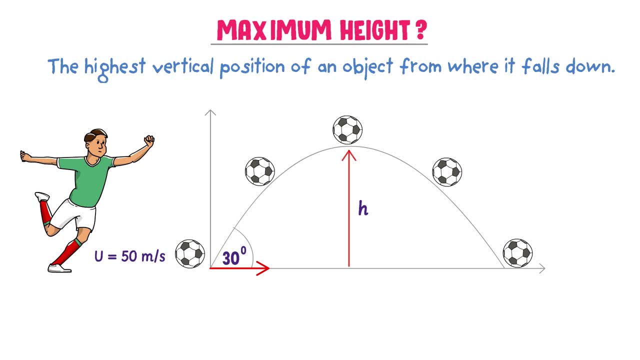 in horizontal direction and its x-component motion is known as the maximum height of the projectile. The y-component of velocity is ux is equal to u cos theta. Also, it moves in vertical direction and its y-component of velocity is uy is equal to u sin theta. Secondly, we learn that at maximum 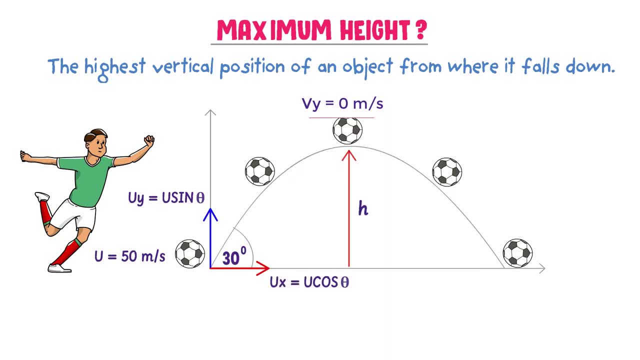 height, the y-component of the initial velocity comes zero, But the x-component of the initial velocity is not zero. If you do not understand all these concepts, then watch the first part of the projectile motion and its link is given in the description. 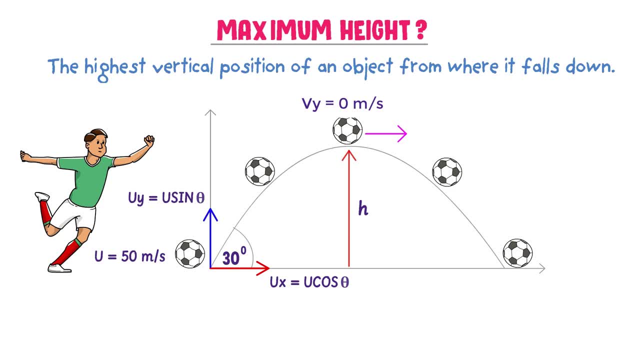 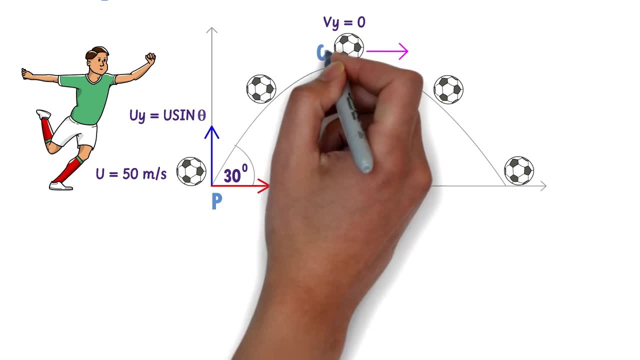 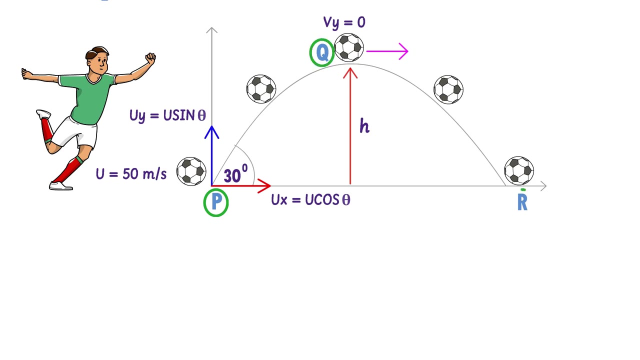 Now I am interested to derive the equation of maximum height of the projectile motion. To do so, I divide the motion of the ball into three points: p, q and r. p is the initial point of the projectile, q is the maximum height of the projectile and r is when the 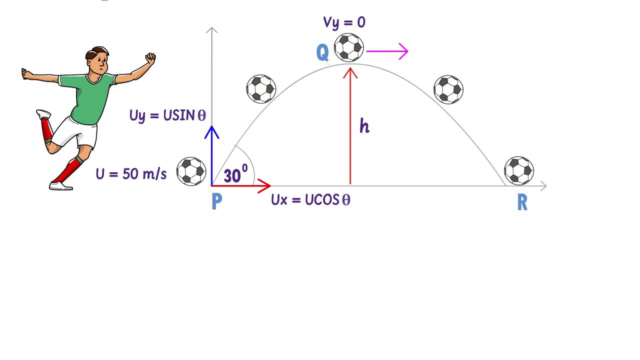 projectile hit the ground. To derive the equation of maximum height, we take the displacement of the ball From p to q and y direction and we neglect the motion of the ball in x direction. We know that the initial velocity of the ball in y direction is uy is equal to u sin theta. 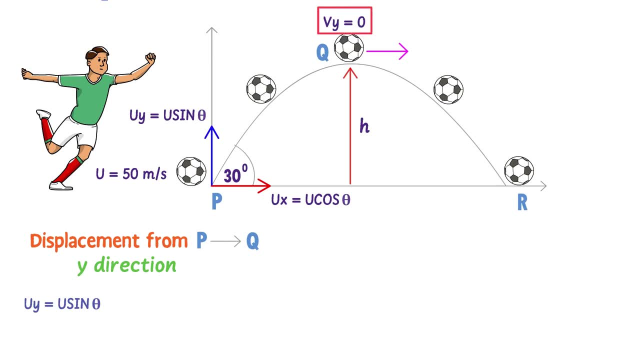 The final velocity of the ball in y direction at point q is: vy is equal to zero meter per second. The acceleration of the projectile is: a is equal to negative g. These all parameters are joined by the equation: 2AS is equal to VF squared minus VI squared. 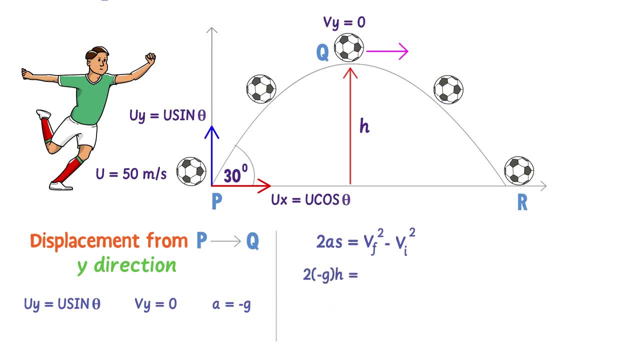 R2 N to negative G N to H is equal to. the final velocity of the ball is 0 meter per second minus and the initial velocity of the ball is UY is equal to U sine theta squared. This negative sign and this negative signs are cancelled out. 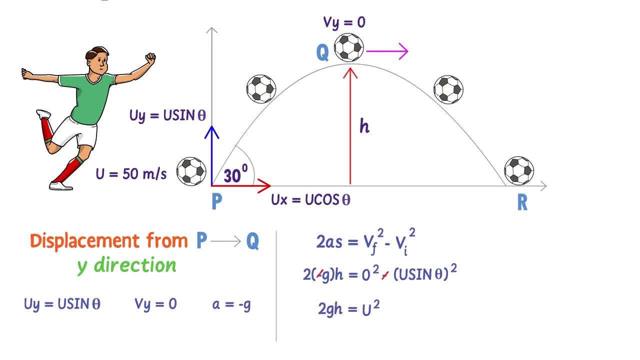 We get: 2GH is equal to U squared sine theta. squared RH is equal to U squared sine theta, squared upon 2G. This is the equation of maximum height of the projectile. Remember that it depends upon sine theta and initial velocity UY of the projectile. 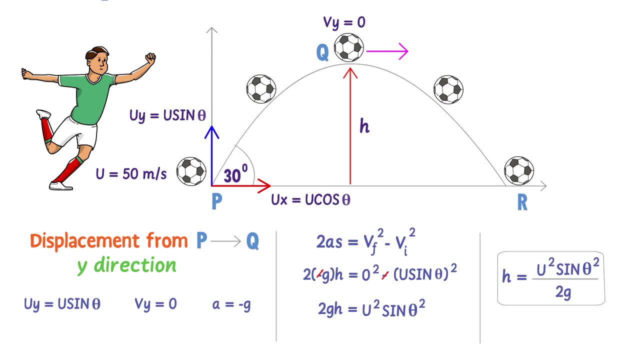 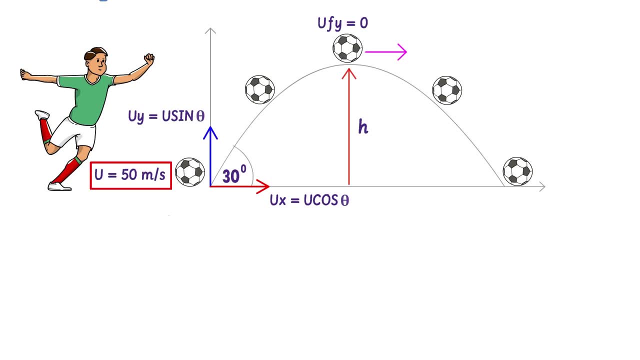 Finally, let me teach you one exam based numerical question. For example, consider that a ball is thrown with a speed of 50 meter per second and a direction 30. Find the height to which it rises. Well, let me write the given data. 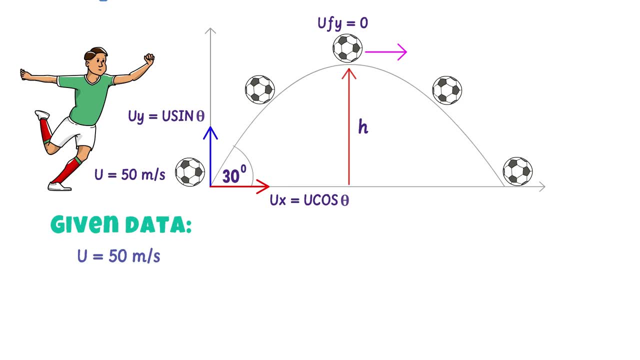 The initial velocity of the ball is: U is equal to 50 meter per second, The angle of the object, theta, is equal to 30 degree and we know that G is equal to 9.8 meter per second squared. The required value is the maximum height, H, of the ball.